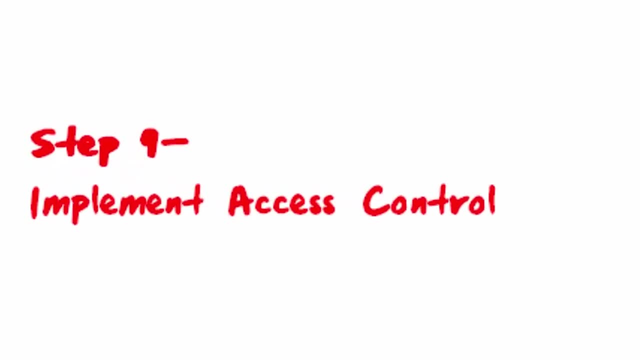 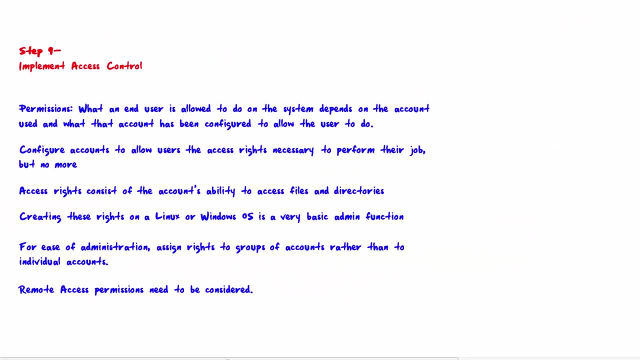 Welcome to Step 9, Implement Access Control. We start with permissions. What are permissions? What an end user is allowed to do on the system depends upon the account used and what that account has been configured to allow the user to do. Most operating systems allow very granular. 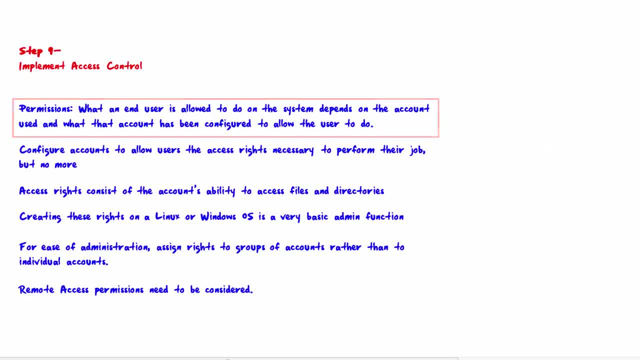 control as to what a particular account is allowed to do. Configure accounts to allow users the access rights necessary to perform their job, but no more. This, if you recall, is the principle of least privilege. Access rights consist of an account's ability to access. 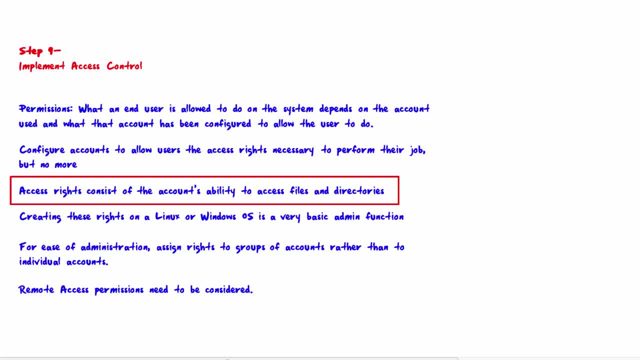 files and directories. If access is granted to a file, is the account allowed to change the file or only read it? If access is granted to a directory, is the account only allowed to read the contents of the directory or are they allowed to create new files in the? 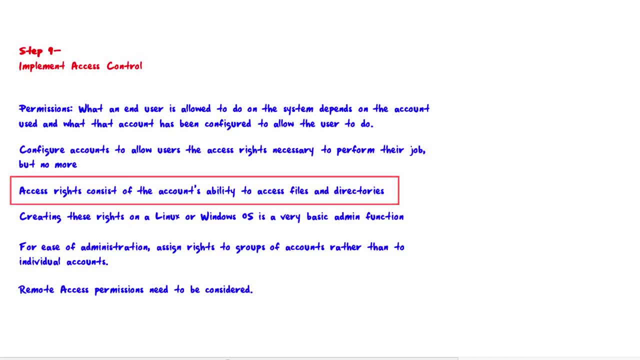 directory, etc. Creating these rights on a Linux or Windows OS is a very basic act- Admin function- So we won't go into the specifics here. For ease of administration, assign rights to groups of accounts rather than to individual accounts. You should create groups of employees with a similar job function and then assign. 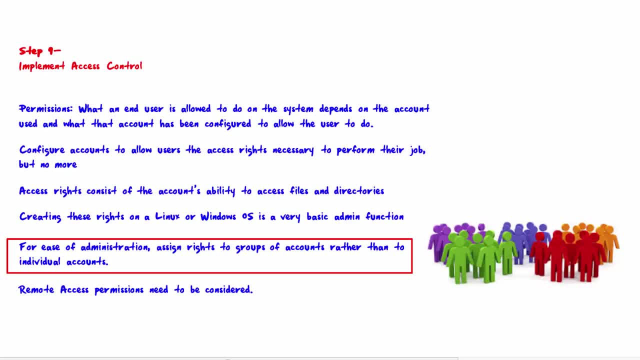 specific rights to the group. For example, all junior accountants will get a specific set of specific rights. For example, all junior accountants will get a specific set of specific set of permissions, while all senior accountants will get a different and probably more permissive. 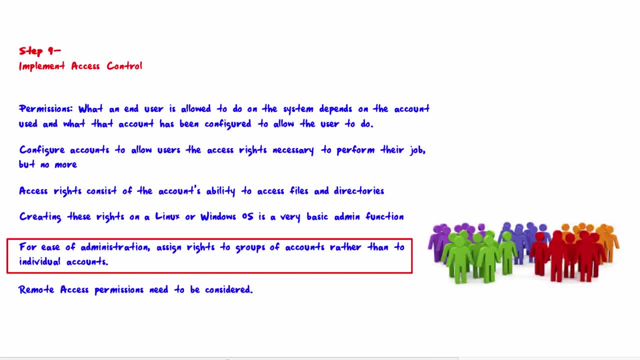 set of permissions. All admin assistants will get a specific set of permissions applicable to their job duties, etc. Remote access permissions need to be considered carefully. That is, if Huckleberry is allowed a specific set of permissions if he is sitting in the home office, is he allowed those very same permissions? if he is?